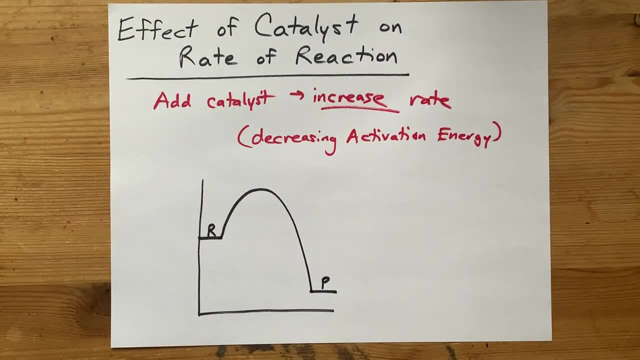 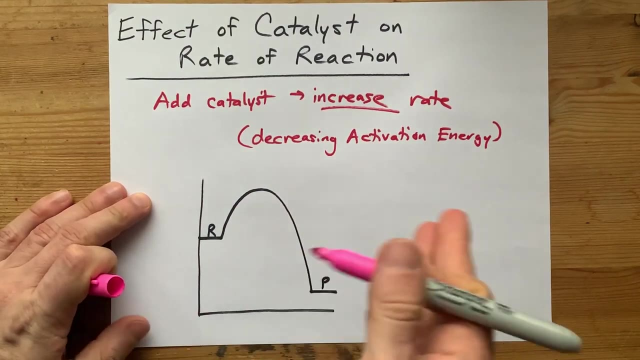 with enough energy to get over the hump. A catalyst provides a new pathway. What I mean is that the reactant isn't just, you know, doing whatever it usually does to create the product. There's a couple of extra steps that are being added. You'll start with the same reactants, but maybe 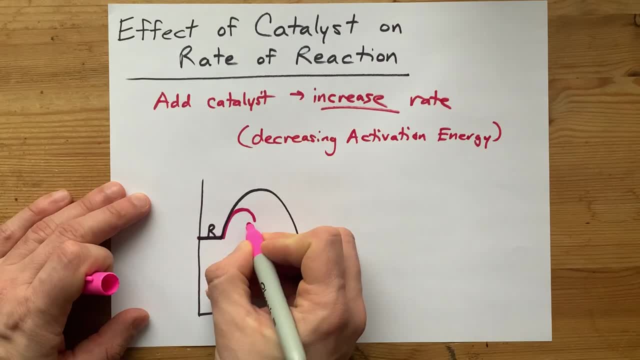 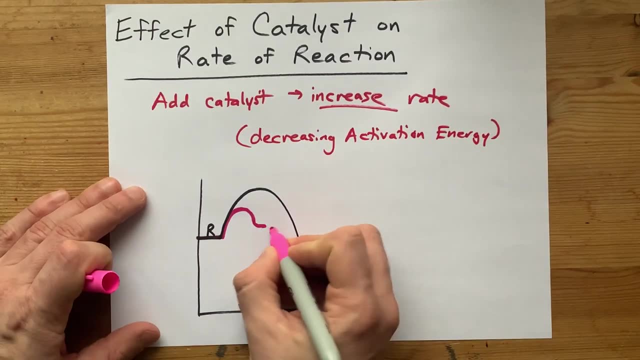 they'll react with the catalyst and that'll be a separate reaction and that gives you some new, new chemical that wasn't present before, And then that new chemical does something else, and at the end of the whole thing you end up in the same place with 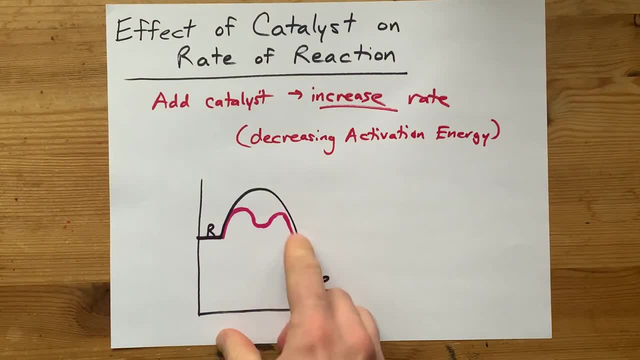 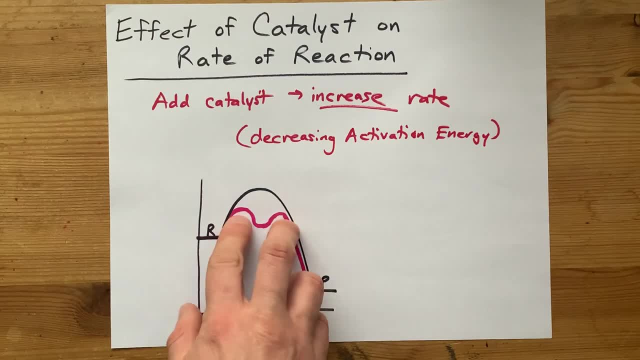 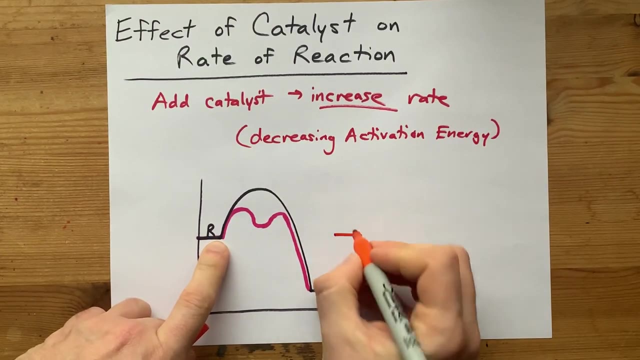 smaller than the original one, And I'm not talking about adding these together, I just mean the threshold, So the amount of energy required to make reactants turn to products with the uncatalyzed reaction Reactants started here and you had to get up to here. The activation energy of the 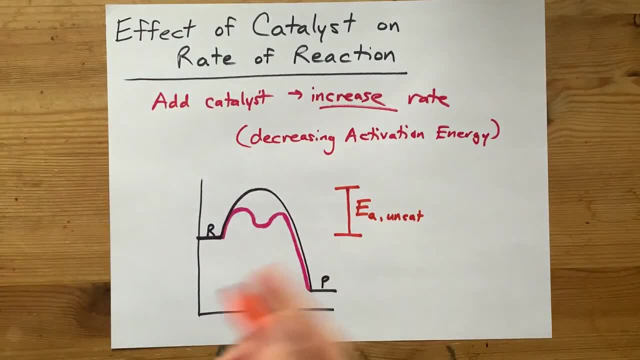 uncatalyzed reaction was this much. I don't know what that is, 70 kilojoules per mole or something. Then for the catalyzed reaction, you started in the same place, but you only had to get up here. 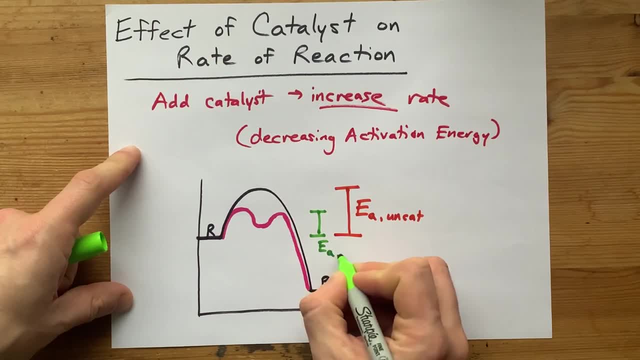 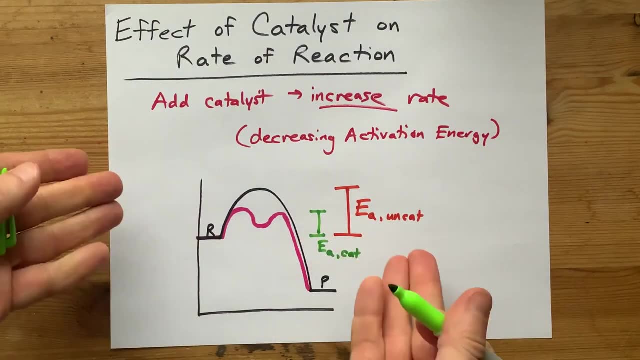 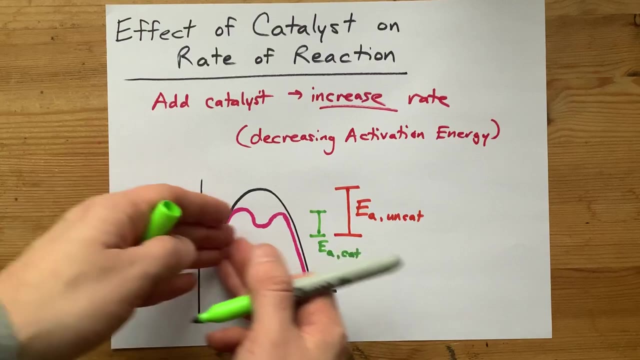 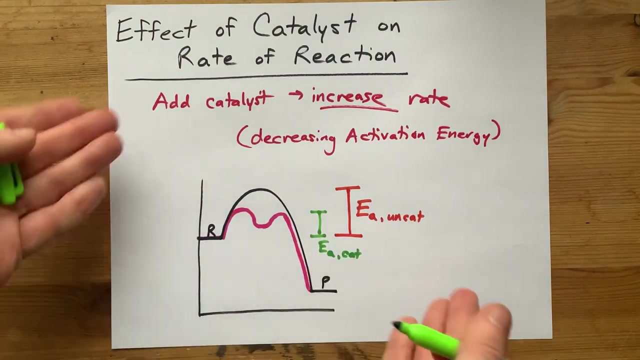 Clearly, that is a smaller amount, And so the activation energy for the catalyzed reaction is less than the activation energy for the uncatalyzed one. What that means is that the uncatalyzed reaction is less than the activation energy for the uncatalyzed one, And that's the 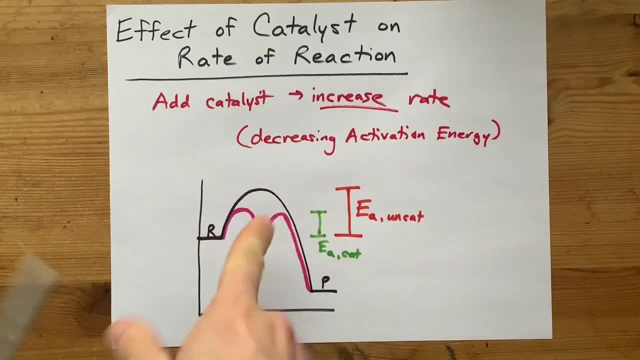 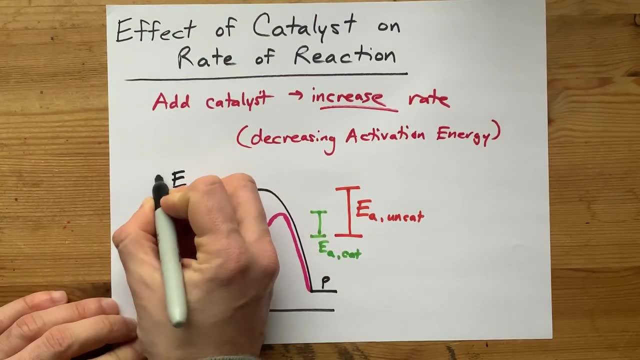 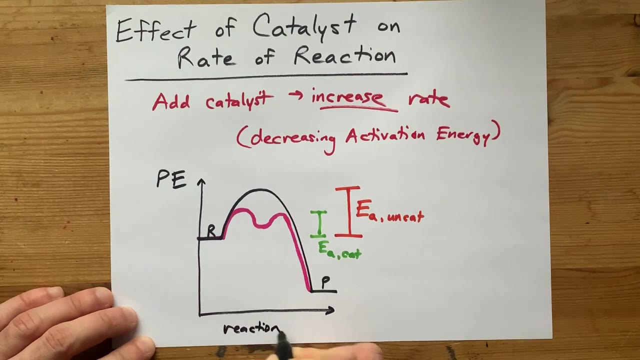 effect of the catalyst. That's the whole thing. Lastly, I'm going to label my axes because your teacher probably wants that too. Some teachers will show this as potential energy PE on the y-axis, And then this is generally like the reaction coordinate where you're starting with. 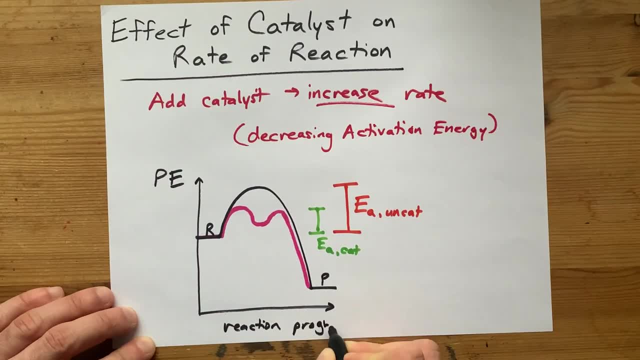 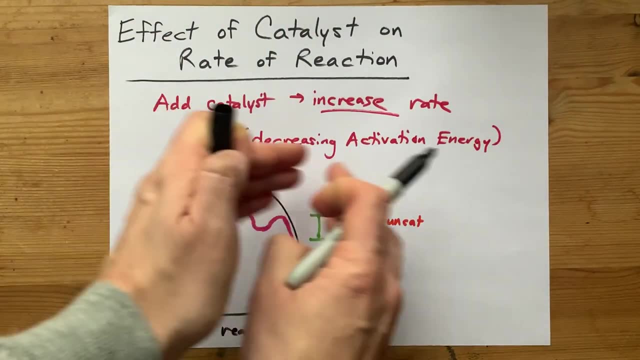 the reaction hasn't started here, and then this is where you finish. You can also label it reaction progress as well. Anyways, the point is, when you add a catalyst, you decrease the activation energy of the overall reaction and therefore the reaction goes faster. You've increased the rate. Great job, Thanks for being with me and best of luck.